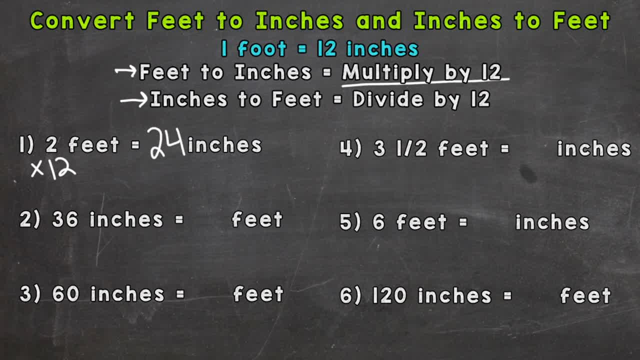 12. And two times 12 is 24.. Again, two groups of 12 inches gives us a total of 24 inches. Number two: we have 36 inches and we are going to feet. So inches to feet, we divide by 12. We're. 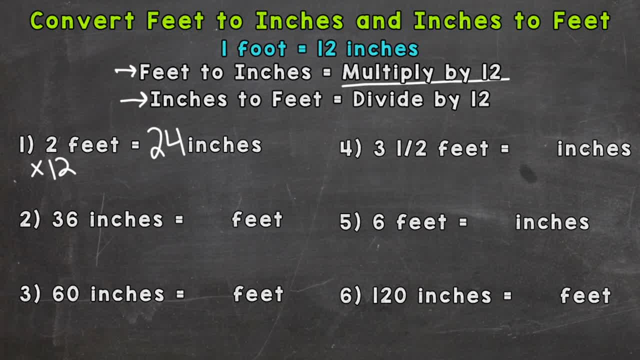 splitting that 36 into groups of 12 or feet. So we need to do 36 divided by 12, which gives us three feet. And again number three inches to feet. So we have 60 inches and we're dividing it into groups of 12.. And again number three inches to feet. So we have 60 inches and we're 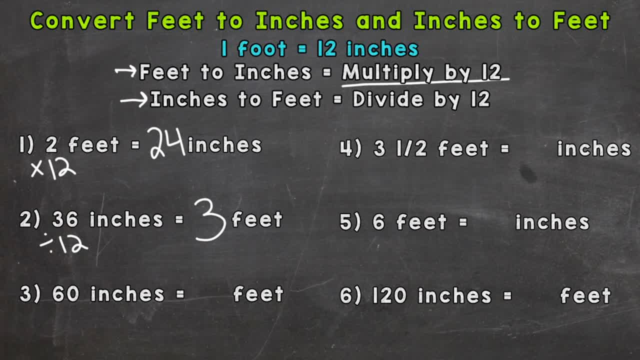 Each one of those groups of 12 is a foot. So 60 divided by 12, you can think of it like this: We're taking that 60 inches and dividing it into rulers, right? Each ruler is 12 inches. 60 divided by 12 is 5 feet. 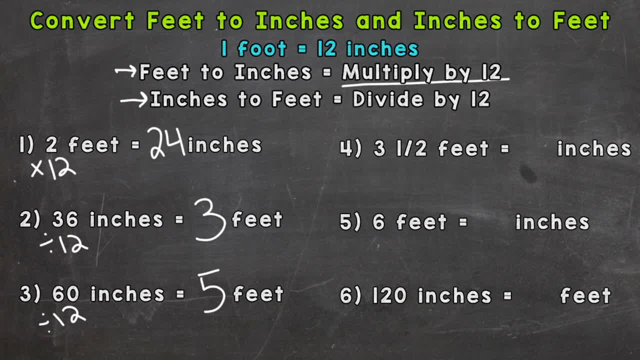 Number 4, we have something a little different. 3 and a half feet equals how many inches? So let's think how many inches is 3 feet? Well, we need to do 3 times 12.. 3 groups of 12.. 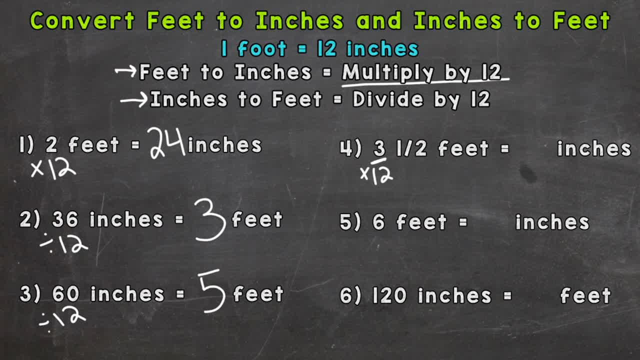 That gives us 36 inches, But that's not going to be our answer, right, We need the half of a foot here, And a half of a foot- well, 12 inches- is one whole foot, so what's half of that? 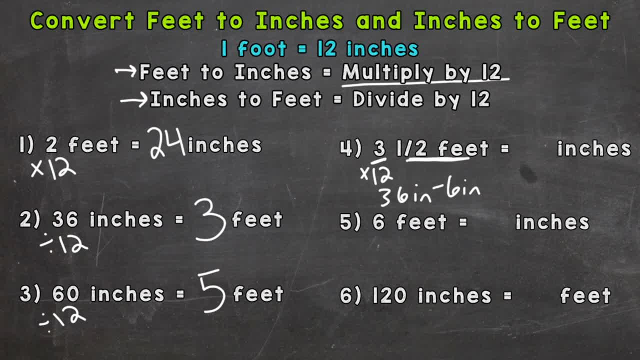 A half a foot is 6 inches, So we need to combine the whole 3 here and the half, So 36 plus 6 gives us a total of 42 inches. So whenever you see a half of a foot, that's 6 inches. 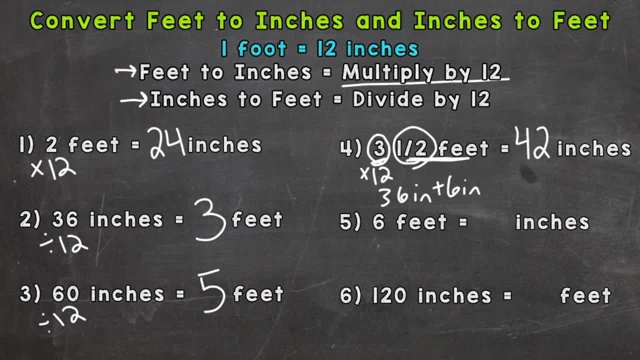 Number 5, 6 feet equals how many inches? Well, we have 6 groups of 12.. We need to multiply 6 times 12, which That is 72 inches. And lastly, number 6, 120 inches equals how many feet?